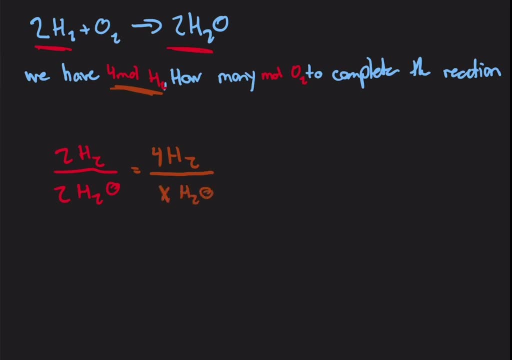 and an unknown amount of H2O. To figure out our X value, we can cross-multiply. We can cross-multiply 2 and X and 2 and 4.. We would be left with 2X equals 8, and after we get rid of the 2 on both, 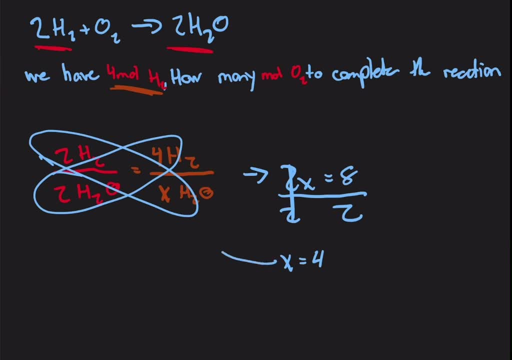 sides, we're left with X- equals 4.. When we plug X back in, we're left with 2X equals 4.. We see that if we have four moles of H2, we will have four moles of H2O. 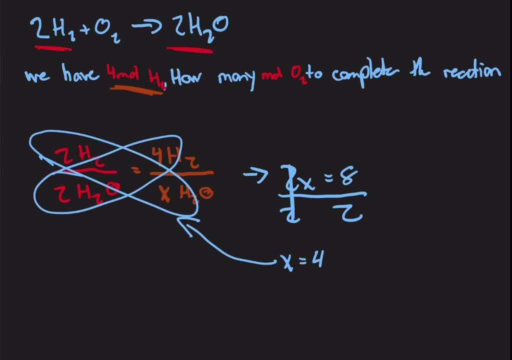 Now that we know how much H2O the four moles of H2 will produce, we need to see how many moles of O2 we need to complete this reaction. We can do this with another mole-to-mole ratio Again. 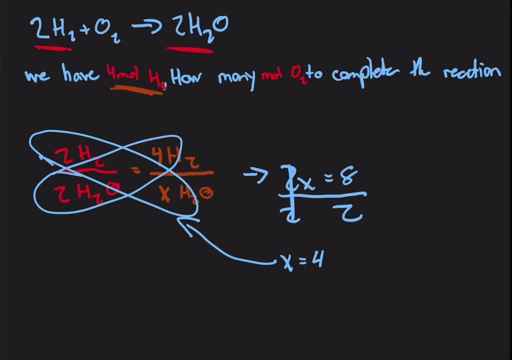 if we were to look in our equation, we see a lone O2 molecule. That lone O2 molecule means one. For every one O2 molecule we get two H2O molecules. We can again write this in a fraction: One O2 will yield two H2O. 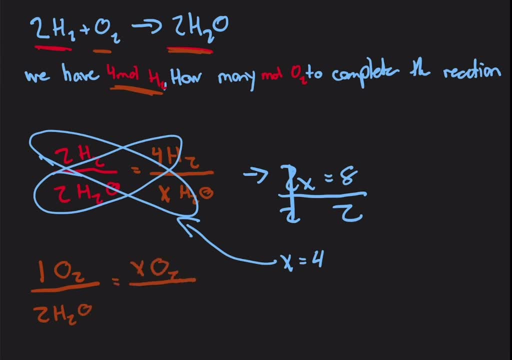 Well, we don't know how many O2 molecules. we need to get four H2O molecules, because that's how much H2O is yielded with our four moles of H2.. Again, we can do some more cross-multiplication with the. 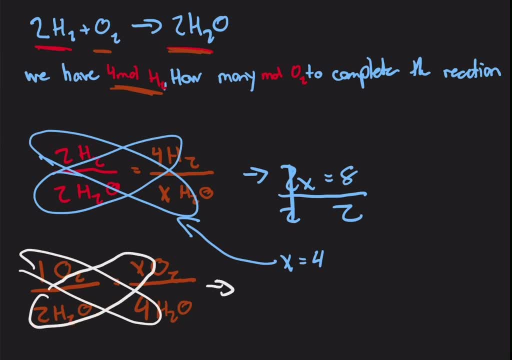 one and the four and the two and the X, We should be left with 2X equals 4.. Again, we divide both sides by 2, and X equals 2.. We can plug that X equals 2 into our mole-to-mole ratio and we can see that. 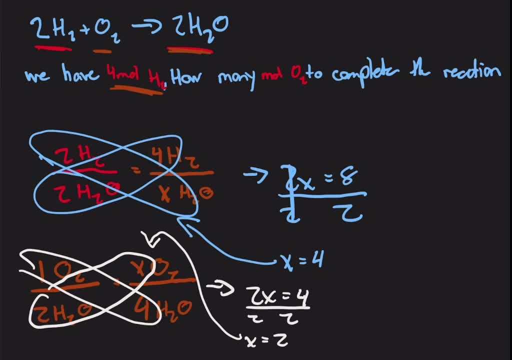 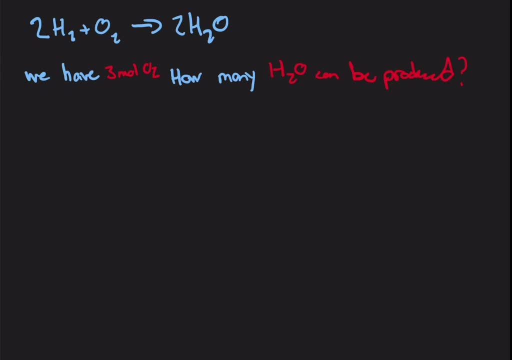 we need two O2 molecules to get us four H2O molecules. We have three moles of O2.. How many moles of H2O can be produced? Pause the video and try this on your own before I reveal the answer. 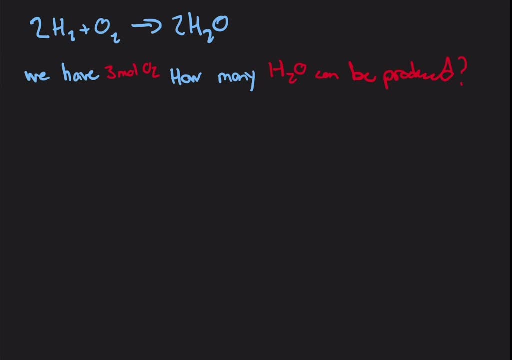 To figure this out, we need to do another mole-to-mole ratio. So for every one mole of O2, we will get two moles of H2O. So let's write that down: One O2 gives us two H2O. Well, we have. 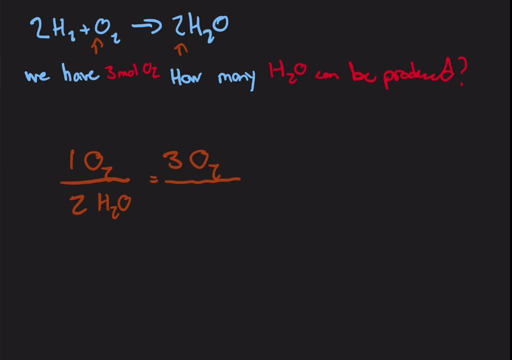 three O2.. We need to figure out how much H2O we get. We can symbolize that with an X. for now, Again, we can cross-multiply the one and the X and the two and the three. that'll give us X equals 6.. We don't need to do any further algebra and we can plug that 6 in. 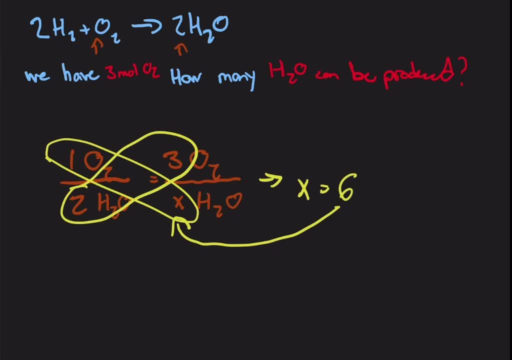 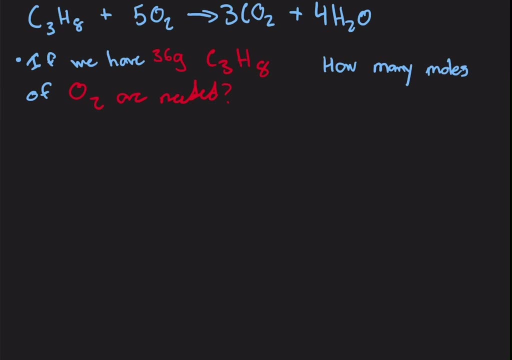 and we know that for three moles of oxygen we would yield six moles of H2O. Let's look at a mass-to-mole ratio. In the last example we did a mole-to-mole example, but now we are given the amount in grams and we need to figure out how many moles are needed. 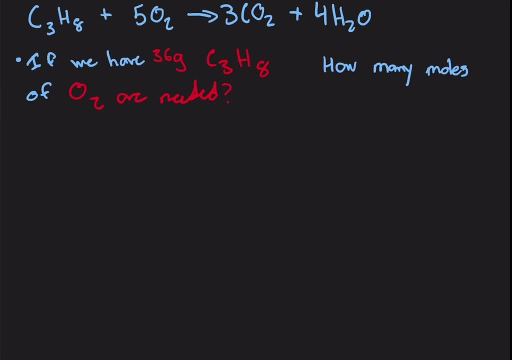 Let's take the equation C3H8 plus 5H2O. C3H8 plus 5H2O yields 3CO2 plus 4H2O or the combustion of propane. We have 36 grams of propane or C3H8, and we need to figure out how many moles of O2 are needed to completely react. 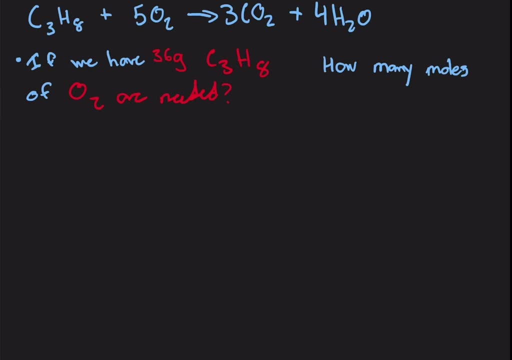 with the 36 grams. Let's do a mass-to-mole ratio to determine how many moles of propane we actually have. So we have 36 grams of propane C3H8. And if we do a mass-to-mole ratio, we want our ending product to be in moles. 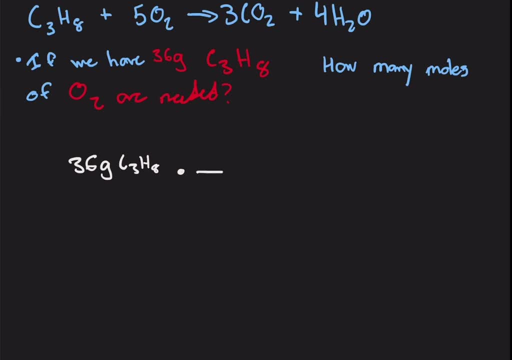 So to cancel out the grams we need to have our grams on the bottom. So the molar mass of C3H8, or propane is 44 grams per mole. So 44 grams of C3H8 is 1 mole of C3H8. 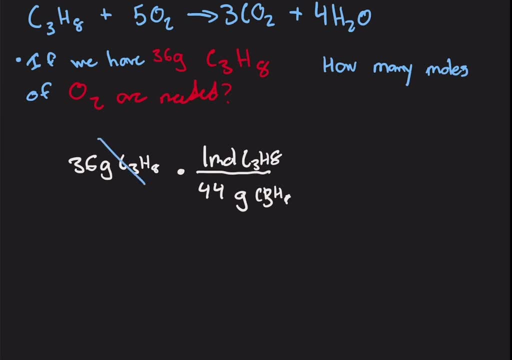 Now, if we cancel out our terms, the grams of C3H8 and the grams of C3H8, will cancel out, leaving us with our unit of moles of C3H8.. And now we need to do 36 divided by 44 to figure out how many moles of propane we have. 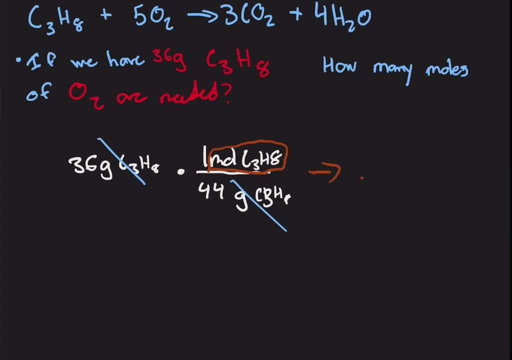 36 divided by 44 gives us roughly 0.82 moles of propane. We now need to see how many moles of oxygen we need to fully react with that propane. To do that, we need to look at the products that are formed: carbon dioxide and water. 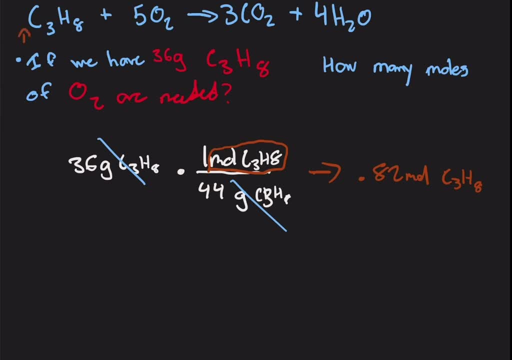 So for every 1 mole, since there's no number here. for every 1 mole of propane, we will get 3 moles of carbon dioxide and 4 moles of water. We can choose either product, since it doesn't specify which one to use. 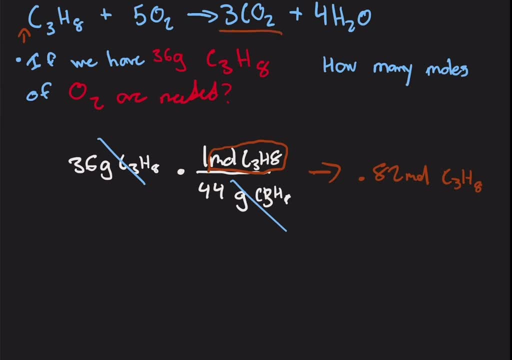 So for this example I'm just going to use the CO2.. So again we can do another mole-to-mole ratio to figure out how many moles of propane we have. How many moles of carbon dioxide are produced from 0.82 moles of propane. 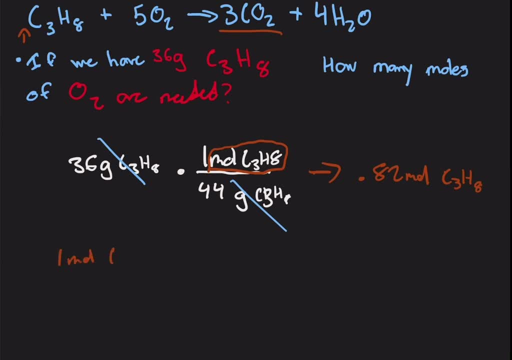 We can set this up by 1 mole of C3H8,, giving us 3 moles of CO2.. And we need to make it proportional to 0.82 moles of C3H8,, yielding us an unknown amount. 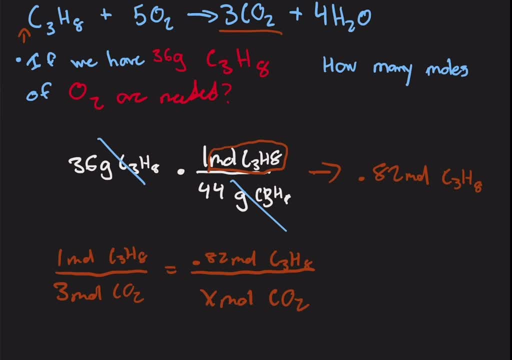 So we have 0.82 moles of CO2.. Again, we can cross-multiply the 1 in the X and the 3 in the 0.82.. This gives us a total of 2.46 moles of CO2. 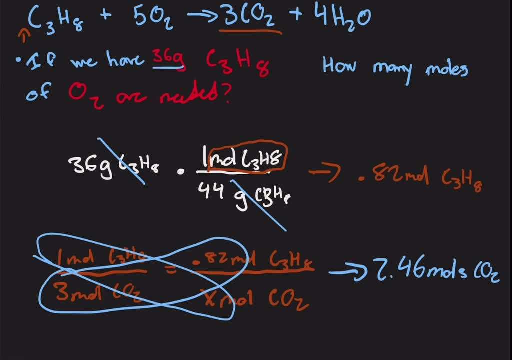 that are formed when we have 36 grams or 0.82 moles of propane. Now we need to figure out how much O2 is needed to make this exact same amount of CO2.. To find out how much O2 is needed to make this exact same amount of CO2,. 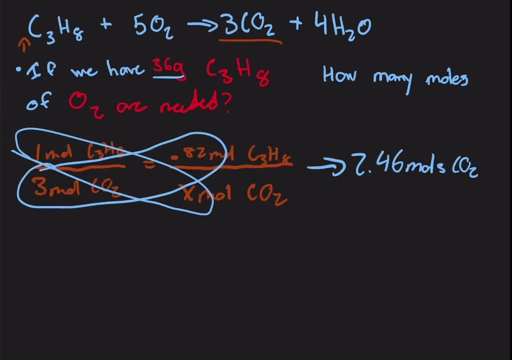 we can do another mole-to-mole ratio. Now, looking at the oxygen, for every 5 oxygen molecules we will get 3 carbon dioxide molecules. If we write this as a mole-to-mole ratio, we have 5 moles of O2,. 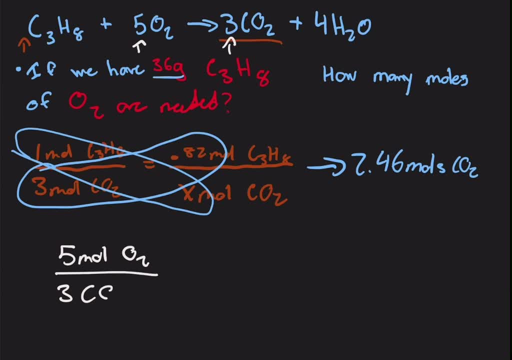 yielding us 3 moles of CO2.. We need to make this proportional to some amount of oxygen which we don't know yet. We'll represent that with an X. That'll give us 2.46 moles of CO2.. 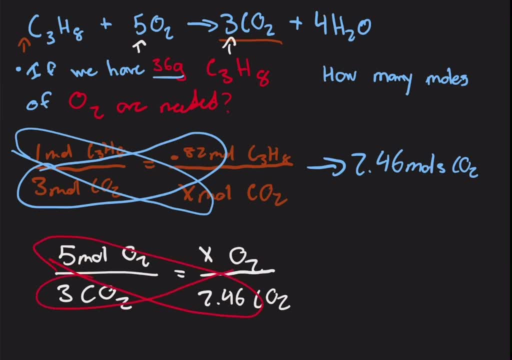 Again, we can just do cross-multiplication to solve for X And we're left with 3X equals 12.3.. After dividing both sides by 3, we get X equals 4.1.. We can plug X back in. 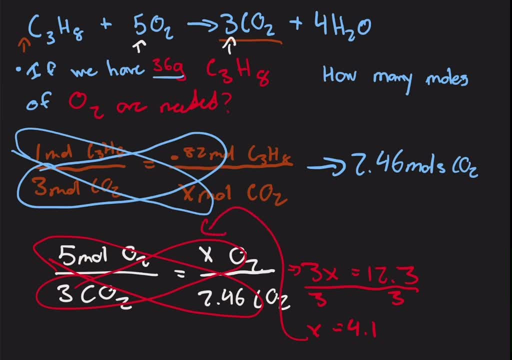 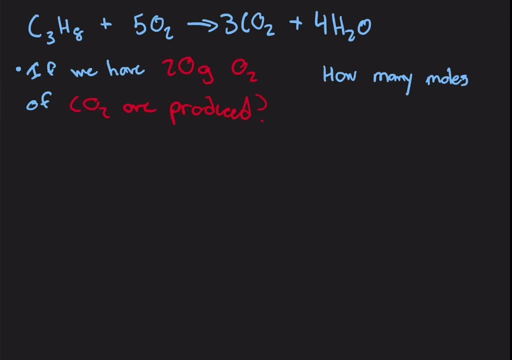 and we can determine that we need 4.1 moles of O2 to yield us that 2.6 moles of CO2.. 2.46 moles of CO2.. Try this equation on your own. Pause the video before I reveal the answer. 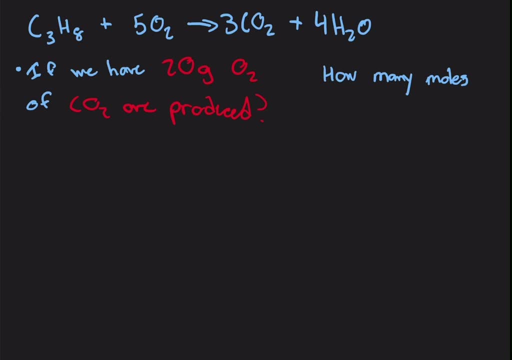 If we have 20 grams of O2, we need to determine how many moles of CO2 are produced. We need to first come up with a mass-to-mole ratio to convert our grams of O2 to moles of O2,. 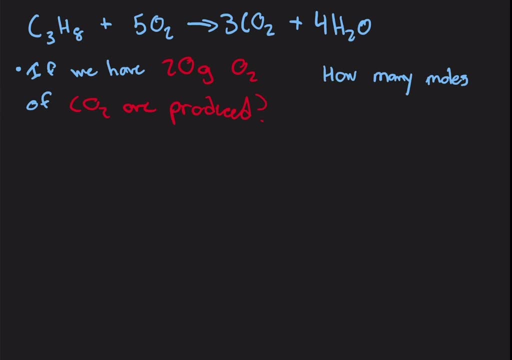 and then a mole-to-mole ratio to figure out how many moles of CO2 are produced. Let's begin with the mass-to-mole ratio. If we have 20 grams of O2, we need to get it to moles of O2.. 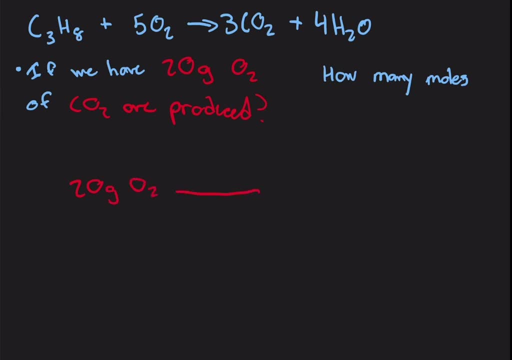 We can do that by putting the molar mass on the bottom in grams and putting one mole on the top. We do this again so the grams can cancel out and we're left with moles. So we're essentially doing 20 divided by 32,. 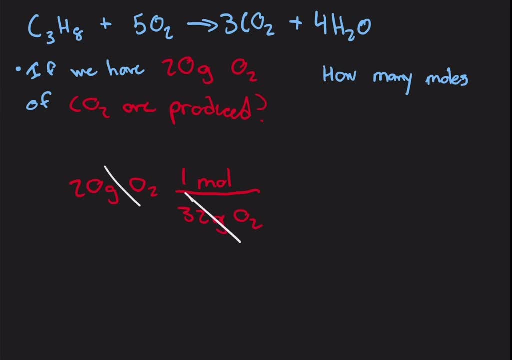 and we're getting rid of the grams to determine how many moles of CO2 are produced. We can do that by putting the molar mass on the bottom in grams and putting one mole on the top. We can do that by putting the molar mass on the top. 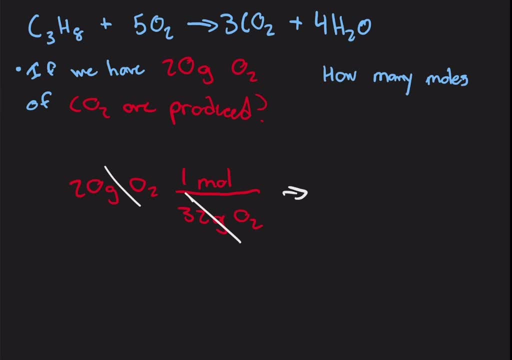 in grams to determine how many moles of O2 we have. 20 divided by 32 will give us 0.63 moles of O2.. 20 divided by 32 will give us 0.63 moles of O2.. 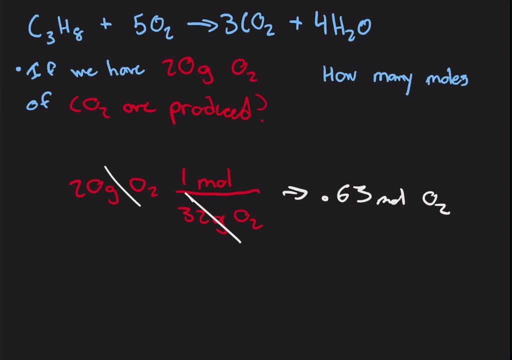 That is what we're working with. We need to see how many moles of CO2 we will make if we put in 0.63 moles of O2 into our reaction. if we put in 0.63 moles of O2 into our reaction. 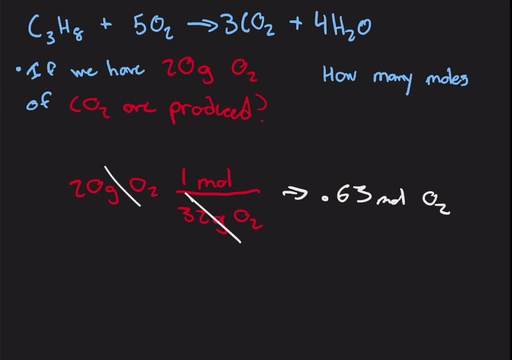 To figure this out, we need to make a proportional mole-to-mole ratio. So we can see, just like our last equation: 0.63 moles of O2 will give us 3 moles of CO2.. 3 moles of CO2.. 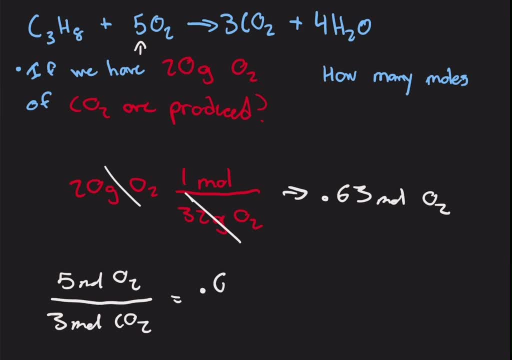 To make this proportional: we have 0.63 moles of O2. we have 0.63 moles of O2 and we have some unknown quantity. and we have some unknown quantity- moles of CO2.. moles of CO2.. 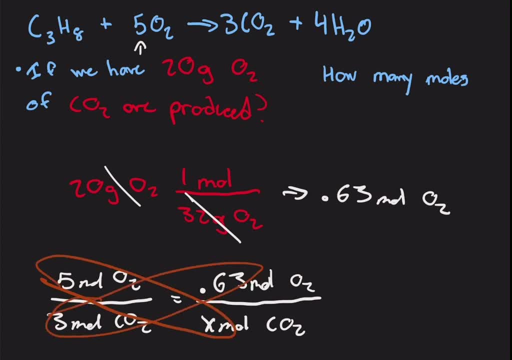 With our cross multiplication. we can multiply 5 and x and 3 and 0.63.. will get 1.89 equals 5x. After dividing both sides by 5, we are left with 0.38 equals x. 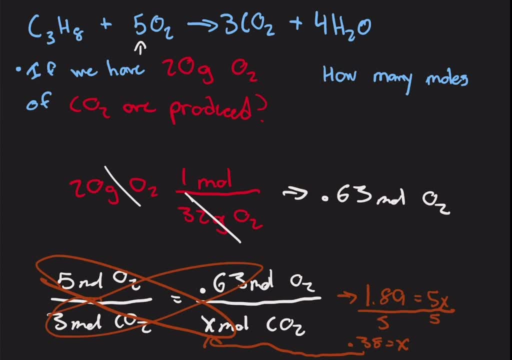 We can plug this in to our proportional mole-to-mole ratio and we can determine that if we have 20 grams of O2, or 0.63 moles of O2, we will get 0.38 moles of CO2.. 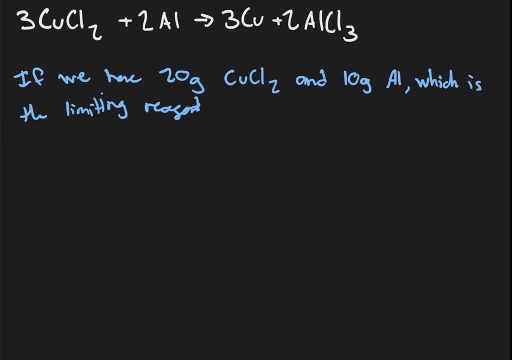 Let's look at a limiting reagent problem In the reaction. 3CuCl2 plus 2Al yields 3Cu plus 2AlCl3.. If we start with 20 grams of copper chloride or CuCl2, and 10 grams of aluminum or Al, 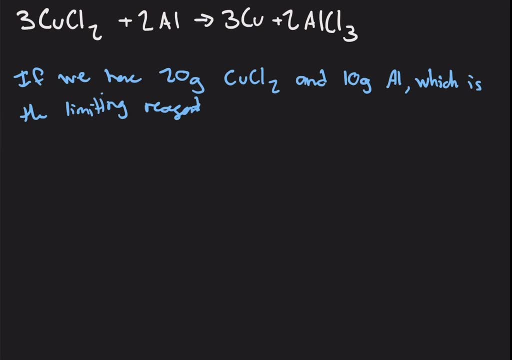 which one is the limiting reagent. So first let's break down what this is asking us. We have 20 grams of CuCl2 and 10 grams of Al. One of these is going to be a limiting reagent, meaning it's going to run out before the other. 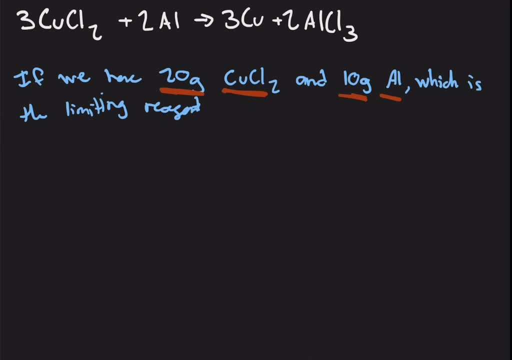 one. To figure out which one this is, we need to determine how many moles of either one of the products will be created from this mass, and whichever one is lower. whichever one produces lower will be the limiting reagent, since it can't make as much as the other one. 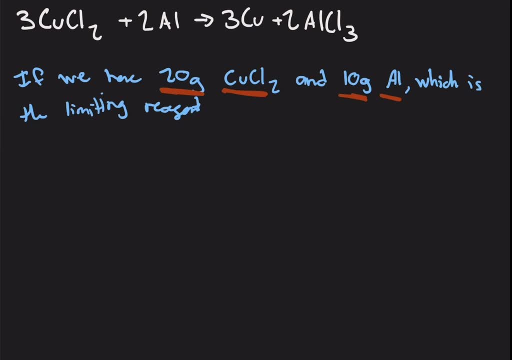 Let's start with copper chloride- CuCl2.. We're going to use a mass-to-mole ratio to convert our 20 grams to the amount of moles. So we can begin with 20 grams of CuCl2 multiplied by 1 mole of CuCl2 over the molar mass, which is approximately 134 grams per mole. 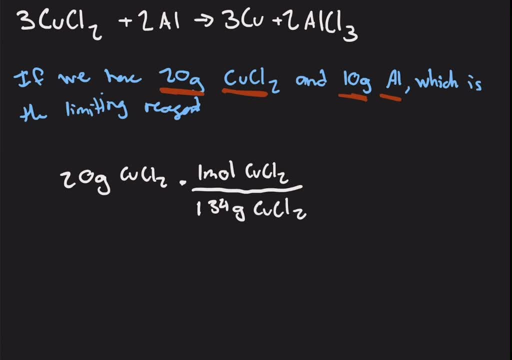 Again, we need grams on the bottom in order for them to cancel out and we're stuck with moles. This is as far as the mass-to-mole ratio is concerned. so we're going to use 20 grams of CuCl2 over the molar mass, which is approximately 134 grams per mole. 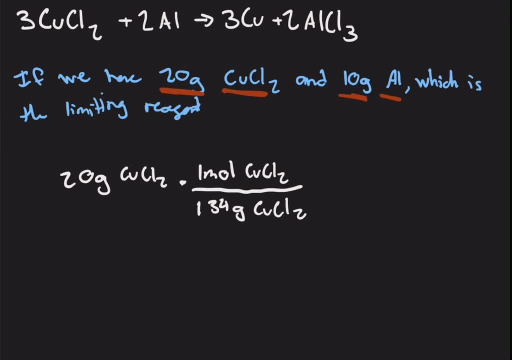 This is as far as the mass-to-mole ratio is concerned. so we're going to use 20 grams of CuCl2 over the molar mass, which is approximately 134 grams per mole. We're going to add a few additional steps. 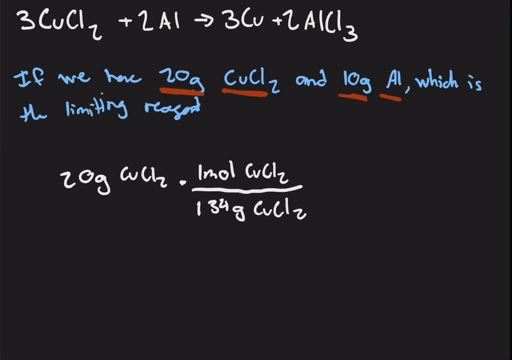 We're going to add a mole-to-mole ratio to this to figure out how many moles of product. What we have right now is telling us how many moles of reactant we have, but we need to figure out how many moles of product that'll create. 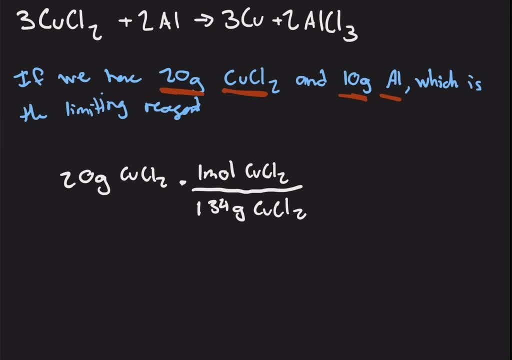 So it doesn't really matter which product we go after. I'm personally going to go for the 3-copper that is created and the mole-to-mole ratio is 3-copper chloride for 3-copper, So it's going to be a 3-to-3 ratio. 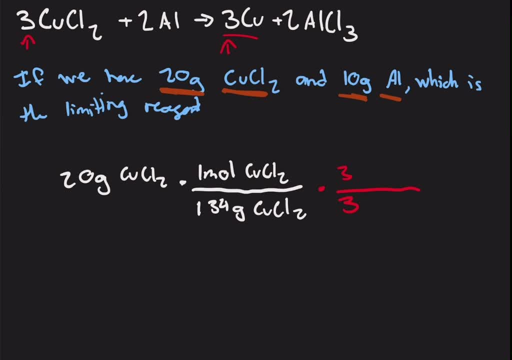 It's important to know which one you put on the top and which one you put on the bottom. We want moles of product, so in this case, moles of copper Cu. We want that on the top because we have moles of copper chloride on the top in the previous fraction, so now we need it on the bottom to cancel out. 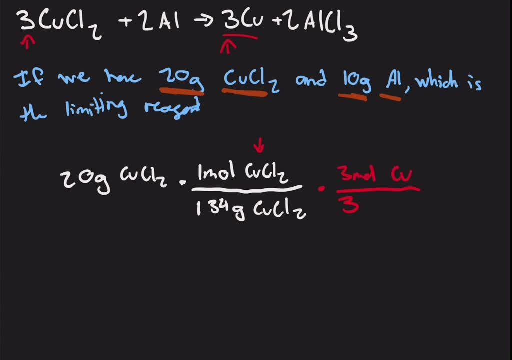 So 3 moles of copper are yielded if we put in 3 moles of copper chloride. Now, if we look at what terms cancel, grams of copper chloride will cancel from the top and the bottom and moles of copper chloride will also cancel from the top and bottom, leaving us only with moles of copper. 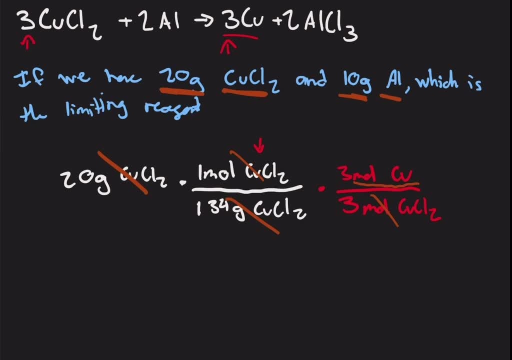 So if we do our 20 divided by our 134, we're left with roughly 0.15 moles of copper chloride, and if it's a 3-to-3 or 1-to-1 ratio, we're also going to have .15 moles of copper chloride. 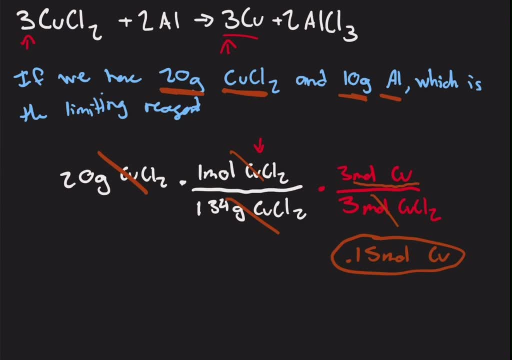 form from this 20 grams of copper chloride. let's do the same thing with our 10 grams of aluminum to see if it creates more or less copper. if we look at our 10 grams of aluminum, we can find the molar mass by putting one mole of aluminum on the top and the molar mass, or 27 grams of aluminum. 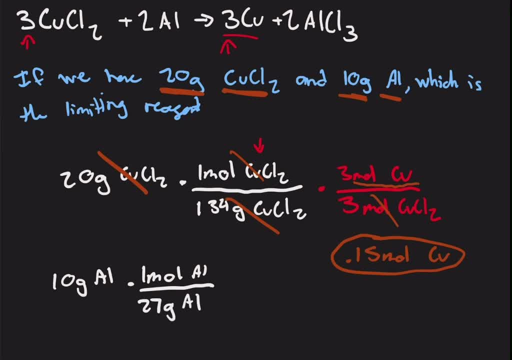 on the bottom. so the grams can cancel out and we're stuck with moles. and now we need to do a mole to mole ratio to figure out how many moles of product will be created. so for every two moles of aluminum we will get three moles of copper. so again we have moles of aluminum on. 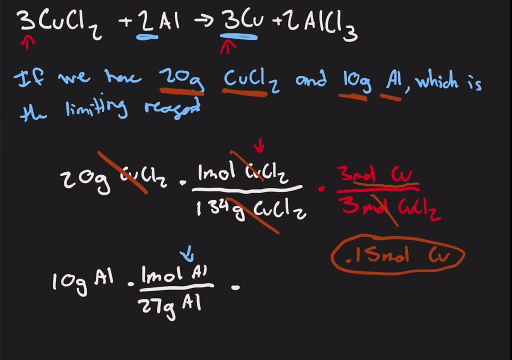 the top. we want moles of copper, so we need moles of copper on the top. so we have three moles of copper that are created for every two moles of aluminum that are put in. let's look at which terms cancel: grams of aluminum, grams of aluminum and moles of aluminum, and moles of aluminum, the only. 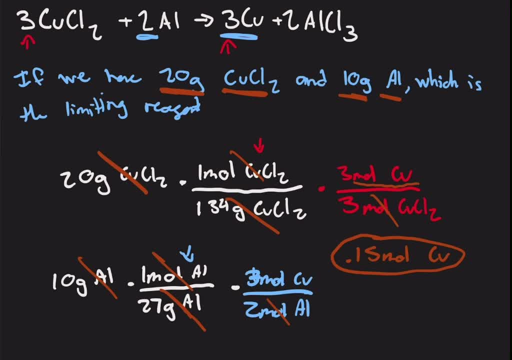 unit that doesn't cancel is the moles of copper, which is what we want. after doing all the math, or 10 divided by 27, multiplied by 3 over 2, we are left with 0.56 moles of cu. this, 0.56 moles of cu. 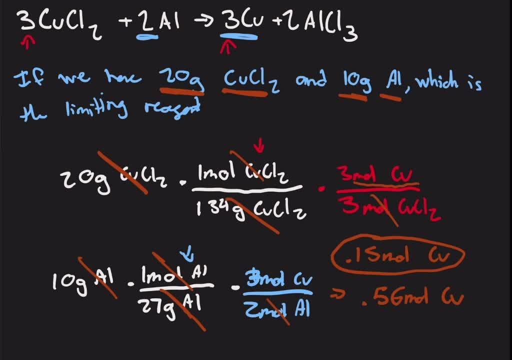 is much greater than our 0.15 moles of cu, meaning that our copper chloride, our cu cl2, is our limiting reagent. with the amount that we're given- the 20 grams and the 10 grams- we can only create 0.15 moles of copper and we are limited from making more because of the amount. 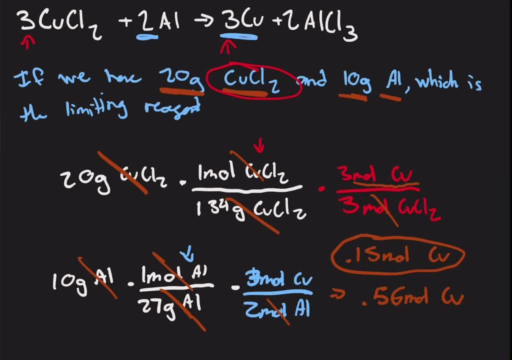 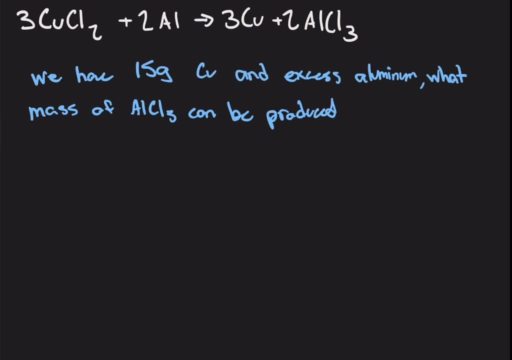 of copper chloride that we have, which is why it is the limiting reagent. try this example on your own. pause the video before i reveal the answer. you: we have 15 grams of copper and excess aluminum. what mass of alcl3 can be produced? so to find the mass of alcl3 that can be produced, we need to determine which one of our reactants 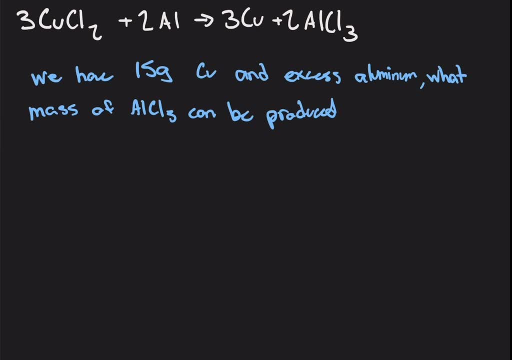 is the limiting reagent. well, in our problem it says we have excess aluminum, meaning that after the reaction is over, we will still have aluminum left over, meaning it is the excess reagent. with that being said, our copper chloride is going to be our limiting reagent in this equation. so we have 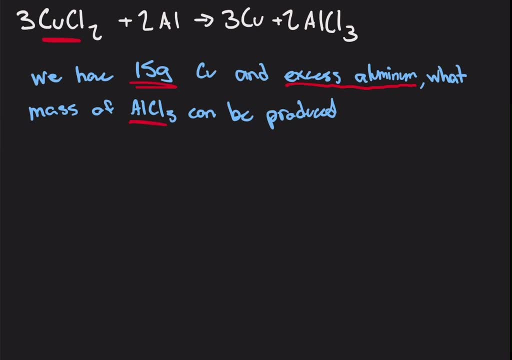 15 grams of copper and we need to figure out how much alcl3 can be produced from that. in order to do that, we need to figure out how many moles of copper chloride produce the 15 grams of copper and then seeing how much that same amount of copper chloride will produce in alcl3 to convert. quoted. 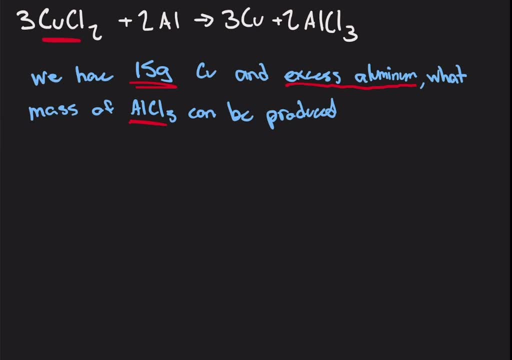 same as put an another line. there is a times $ 105 million when почick order of Cu and 6% in Cu by a result of the piÄôlar and mu light have each other. that has calculated the first distance to the. To convert grams of copper to moles of CuCl3, we first need to do a mass-to-mole ratio to get the moles of copper. 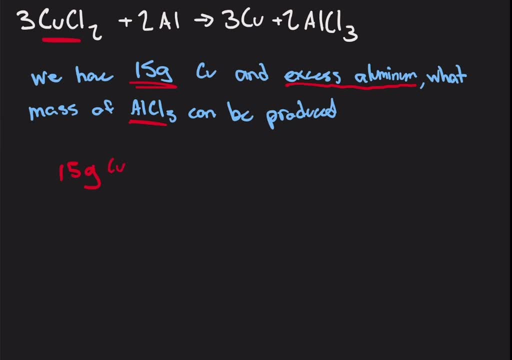 Well, we have 15 grams of copper multiplied by 1 mole of copper and the molar mass, which is roughly 64 grams of copper. Again, grams are on the bottom, so they can cancel since they're on the top in the 15 grams. 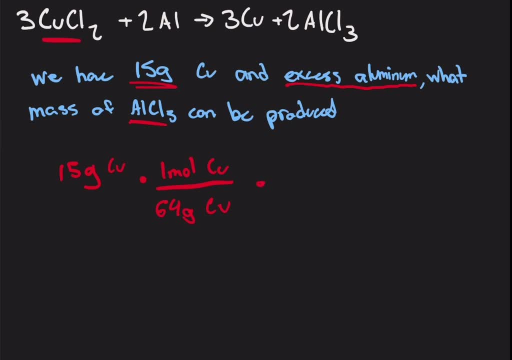 And then we need to do a mole-to-mole ratio. Well, like we said previously, 3 moles of CuCl2 will yield 3 moles of Cu, So it's a 3-to-3 or 1-to-1 mole ratio. 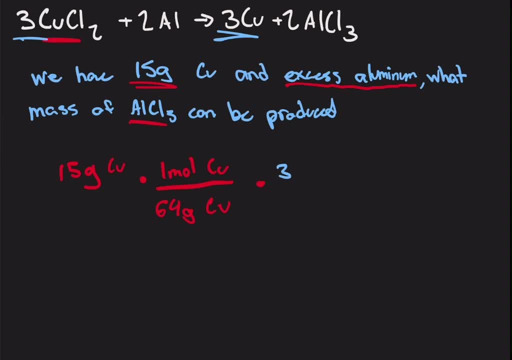 So we want moles of CuCl2 as our final product, so we're going to put it on the top, because we have moles of copper on the top here. We need it on the bottom, so they cancel out. So we'll put 3 moles. 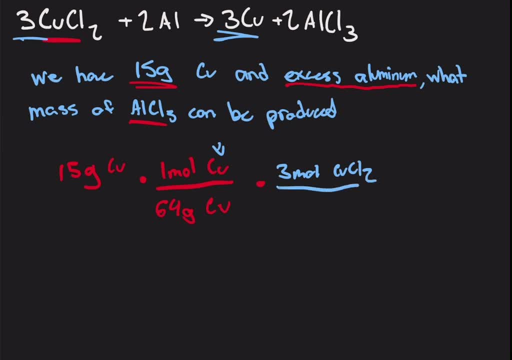 Moles of CuCl2 over 3 moles of Cu. Let's see which terms cancel. Our grams of copper will cancel, and then our moles of copper will cancel. After doing our algebra, we're left with roughly 0.23 moles of CuCl2.. 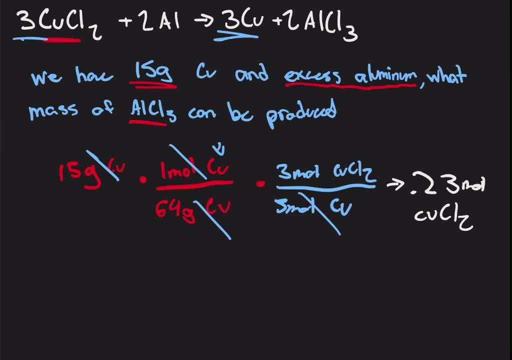 And now we need to see how many moles of AlCl3 this amount of copper chloride will produce. So we're going to do the exact same thing, except we don't need a mass-to-mole ratio this time, since we're already working with moles. 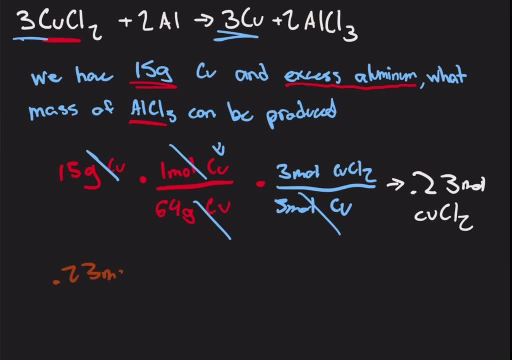 So if we have 0.23 moles of CuCl2, it's going to give us an unknown value of AlCl3.. But we do know that 3 moles of copper chloride will give us 2 moles of AlCl3. 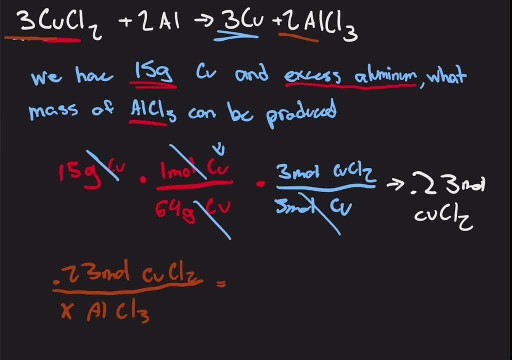 2 moles of AlCl3. So we can write that down and find a proportional fraction. So if we put 3 moles of CuCl2 on the top and 2 moles of AlCl3 on the bottom, we can once again do cross-multiplication with the 0.23 and the 2 and the x and the 3 to determine what our x value is.